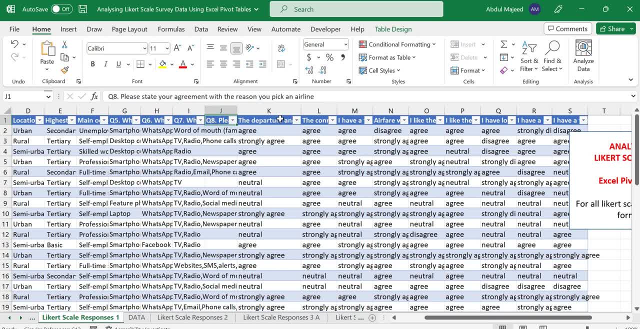 where we ask respondents to read: give their responses for regards to agreeing or disagreeing to a certain statement. So we want to summarize all these statements, within the lack of skill responses, in a single chart and be able to compare which statement do respondents strongly agree or they? 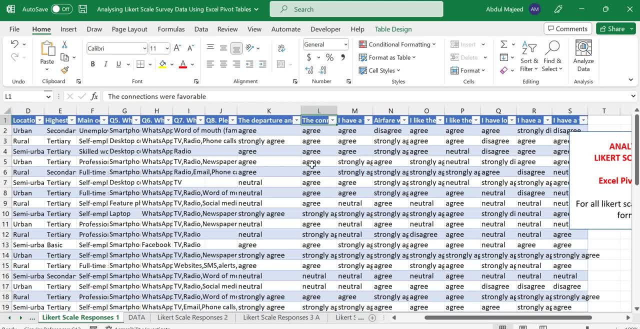 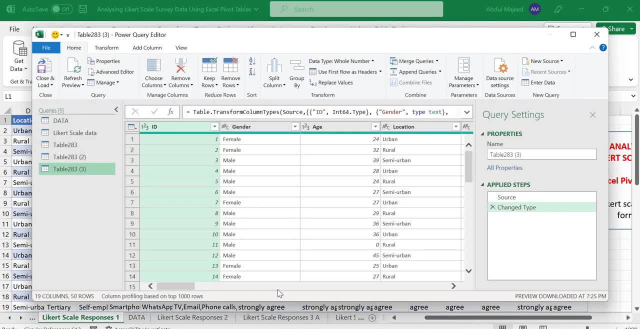 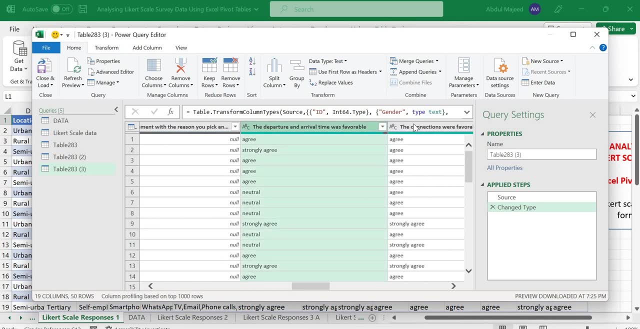 agree or they associate with, and so on. so how do we handle this? so first you need to load your data to power query. so once you load it to power query, the next thing you need to do is the next thing you need to do is to select all the the columns with the statement that you want to summarize. 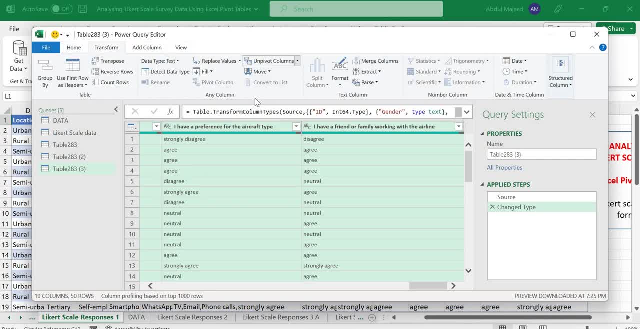 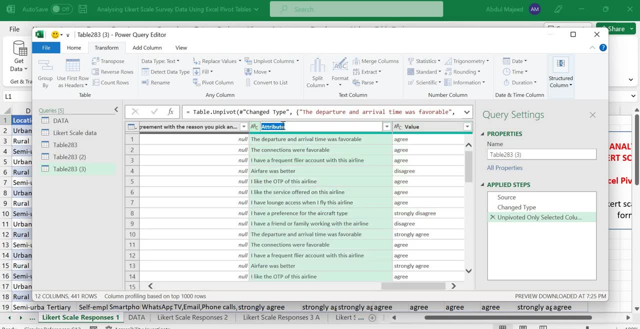 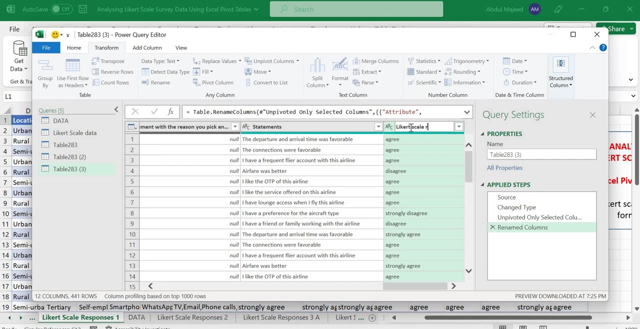 so once you do this, you go to transform from transform to unpivot only selected forms. then we have it here, so this attribute column can name it. then here, uh, the value column, the lax scale sponsors, all right. so once we uh, we have this, we are done. so we go to home from home. 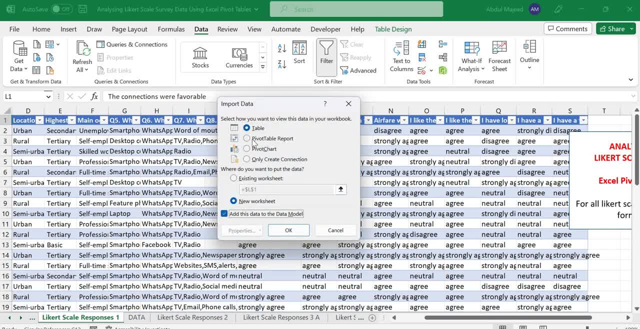 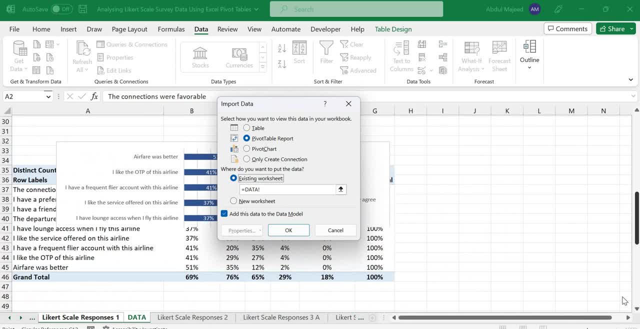 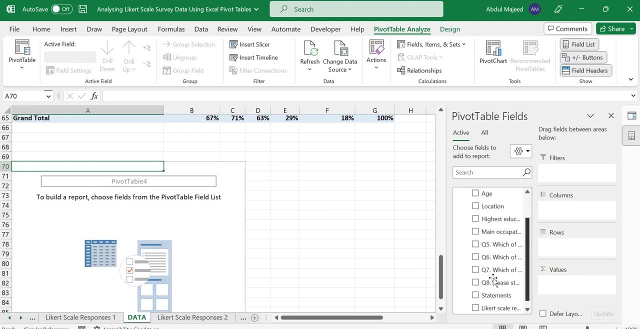 uh, load this uh and add it to the data model. we want to generate a pivot table in our existing sheet, so we want add a pivot table in this shape. Alright, and we have it. We want to compare the statements by how many people who agree or disagree to each of the 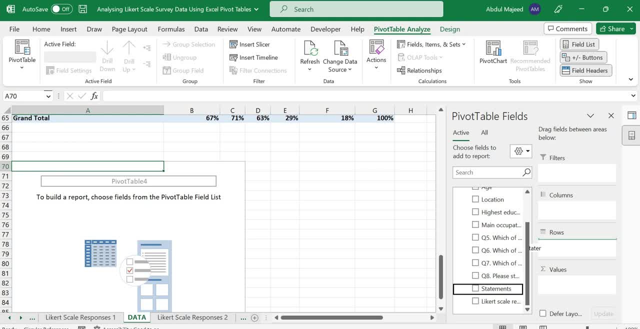 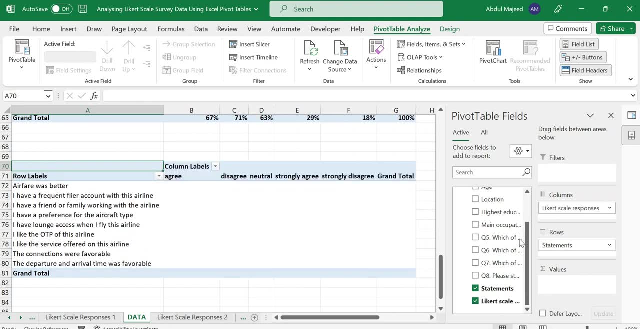 statements. So we pick the statement and put the statement and then drop it in the row. first We pick the responses and drop it in the column first, and then we want to count each statement by the Lekesql responses. So we pick our ID and drop it in the value first. Now by default, because the IDs are 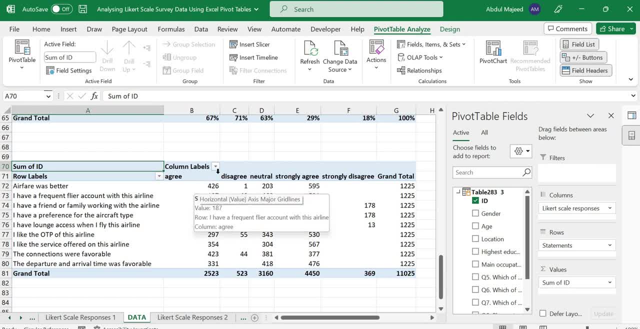 memory Pivotable summarizes by sum, but we want to have the responses by count. So let me clarify something. There are different ways people can handle Lekesql, but the most common approach depends on how you kind of consider your data. So some 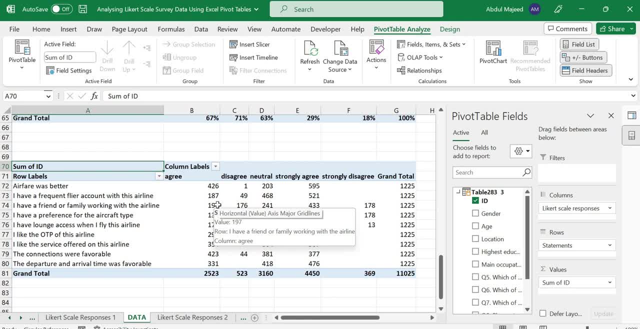 treat Lekesql as an ordinal data, others also treat it as interval data and this will all kind of influence have an impact on how you handle your data. We wouldn't go into that argument. The thing is that if your objective- that initiated or that led to the use of the Lekesql- is to see 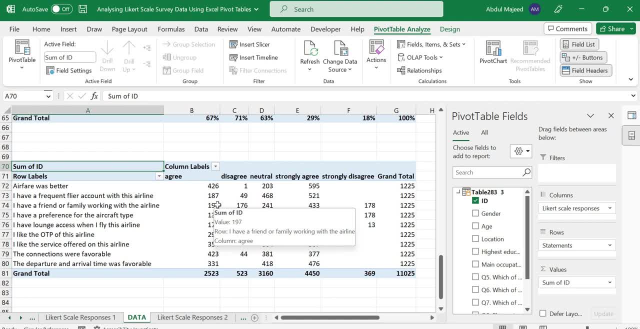 the distribution of responses across the scale. then you just use proportions. That means treating your data as an ordinal data. In the most common summary statistics you can handle you can apply, for this are just a counts, and then you take proportions or you also look at the mode We are looking at. 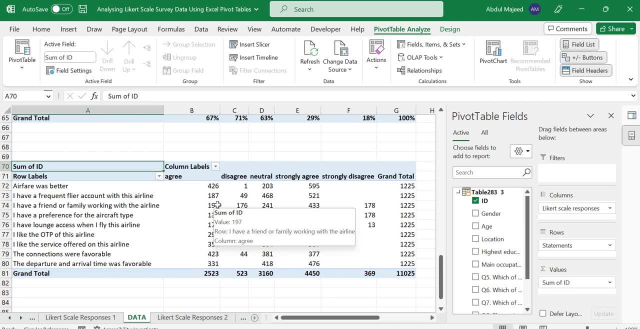 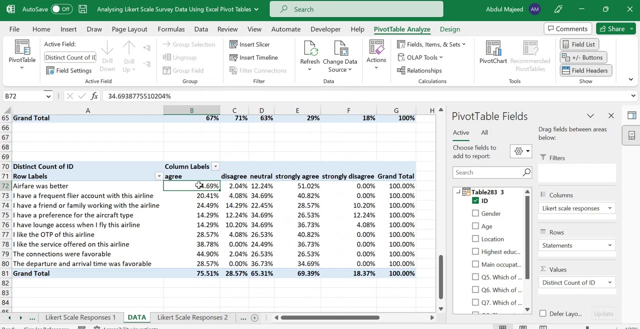 a proportion where we just want to look at how the responses are distributed across that scale. So here we right click and then summarize by distinct count to get the exact number of respondents who selected each label for each statement. So we then take the percentage by row. 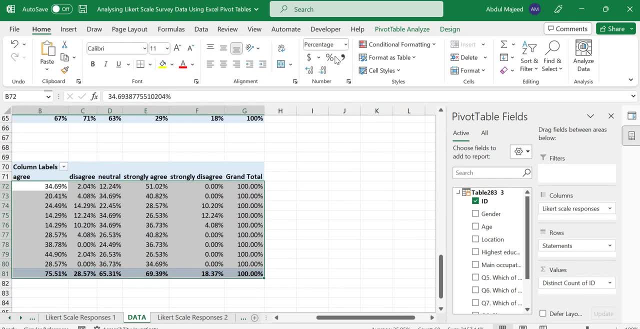 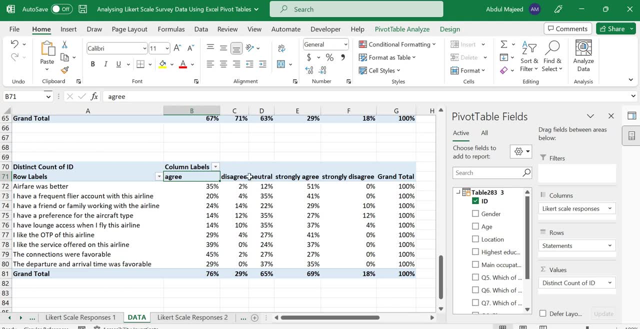 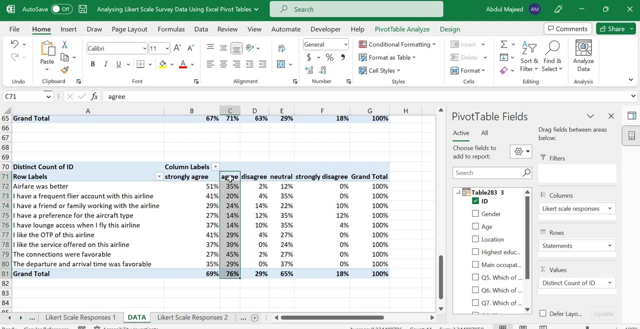 For each statement. we want to see how many of the respondents agree, disagree, so on. So once we have this, what we can do is that we can arrange our scale in descending order. So we have strongly agree, agree, and we can bring neutral next. we just shift it then. 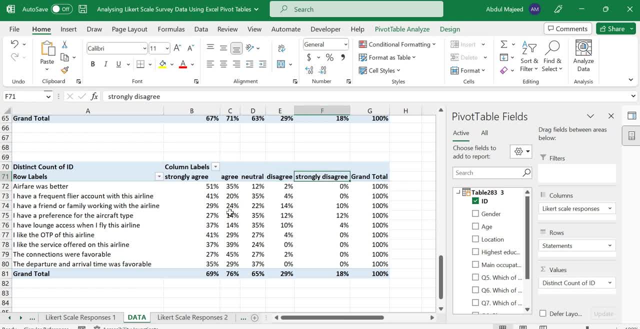 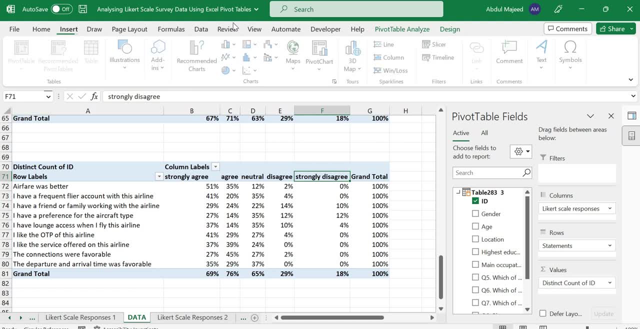 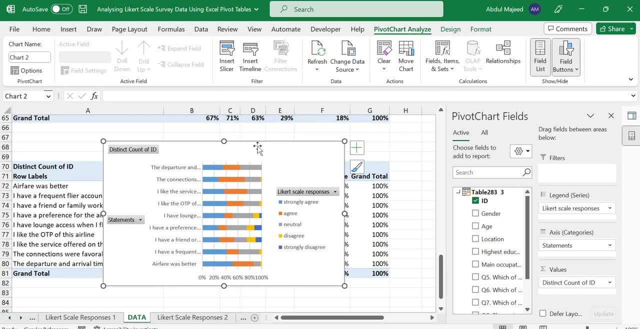 we have. the next thing is disagree and then strongly disagree And then that's it. I've summarized to make a scale using a pivot table So you can insert a chart. they are appropriate because each statement add up to half. So if you have 100, you can use stack-by-chart. 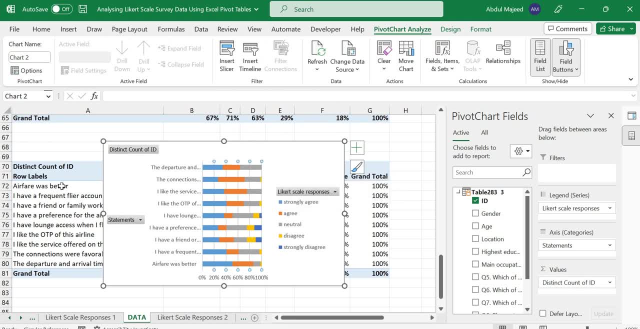 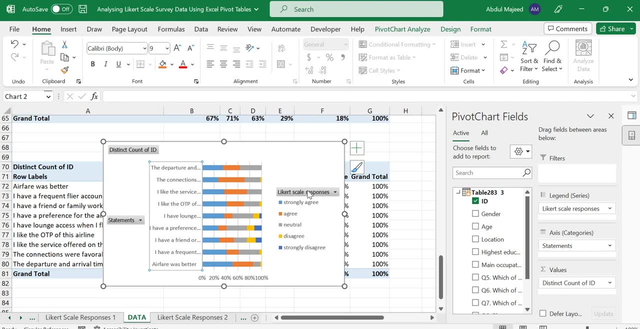 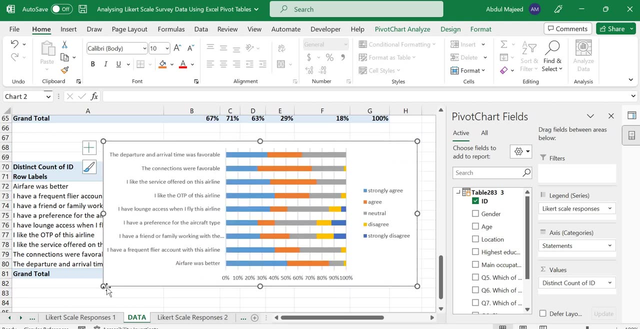 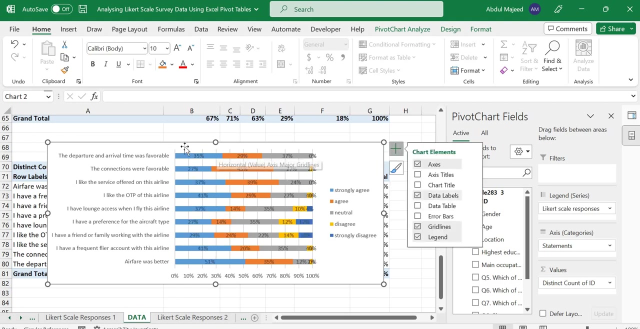 Now we are choosing a horizontal stack-by-chart because our statement takes quite longer, So it will be more convenient to use a horizontal stack-by-chart. That will be able to show all the labels and you can resize your data appropriately. All right, So once you have this, you can just add the data labels- percentages. 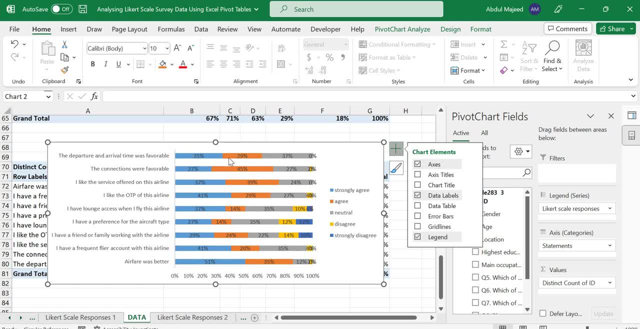 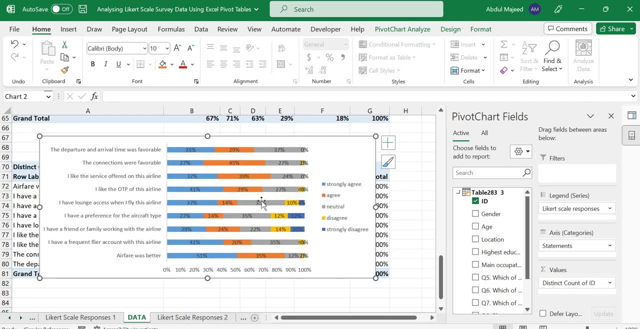 You can Format this chart, make it look very, very nice, so on. So that is it, And we are done, Thank you.